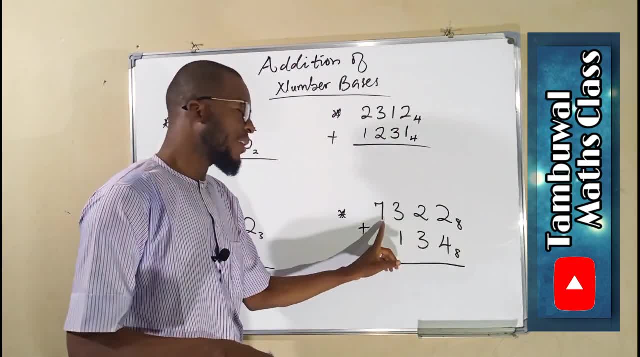 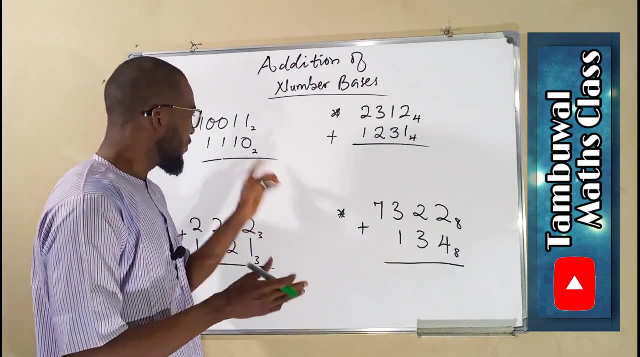 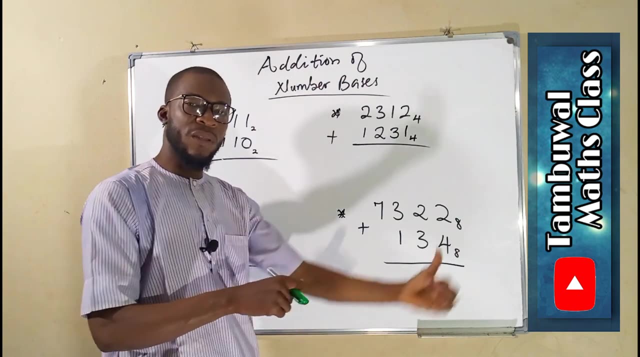 is 4. we do not have 4. this is 8. the highest we can have is 7. so, as you are asked to add a number or combination of those numbers reach the base or greater than the base, all you have to do is to keep down the remainder and take the. 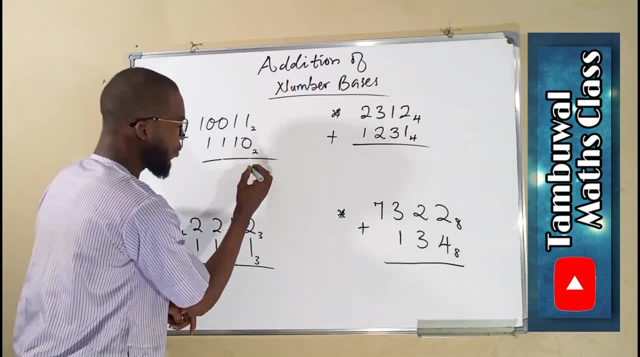 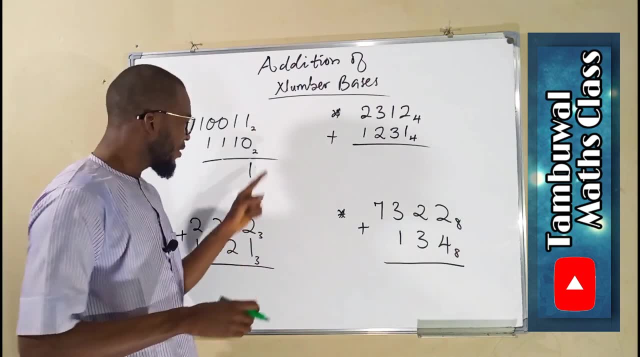 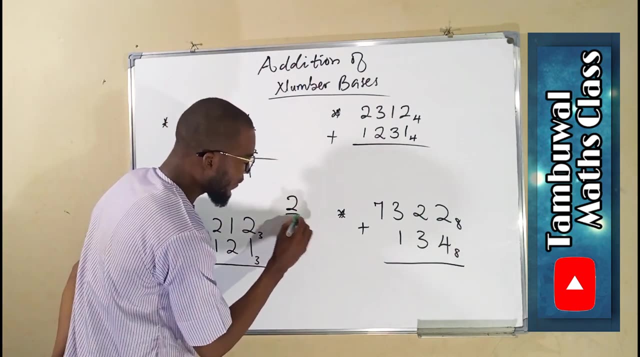 other digit to the next level. 1 plus 0 is 1 and 1 is less than the base. 1 plus 1 is 2, but 2 is exactly the same as the base. so we have to take down the remainder 2 divided by 2. 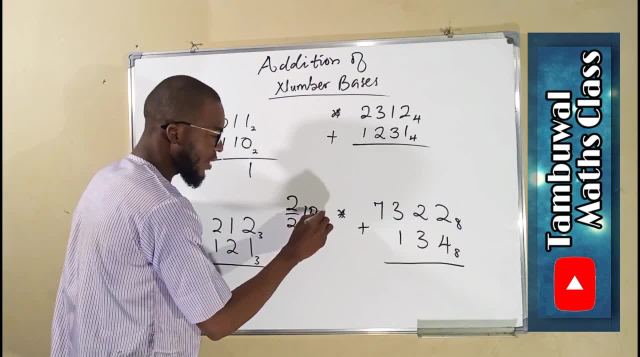 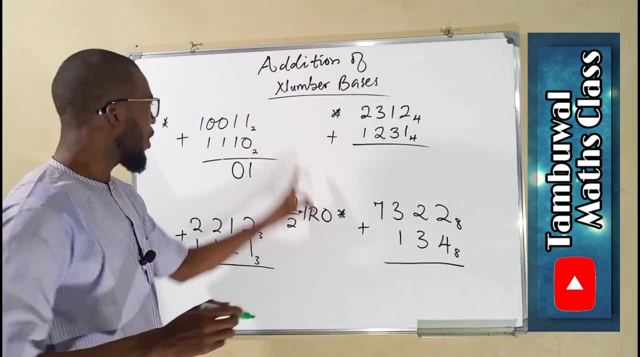 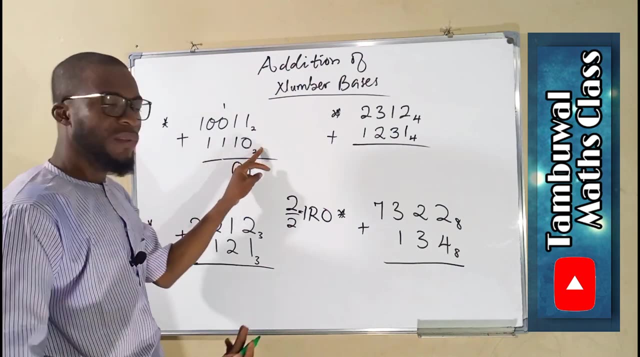 we can go into 2 one time, remainder 0. so we keep down the remainder, which is 0. then we take that 1 to the next level. 1 plus 1 is the same thing as 2. 2 is the same thing as the base. so we divide 2 by 2, we have 1 remainder 0. write down the. 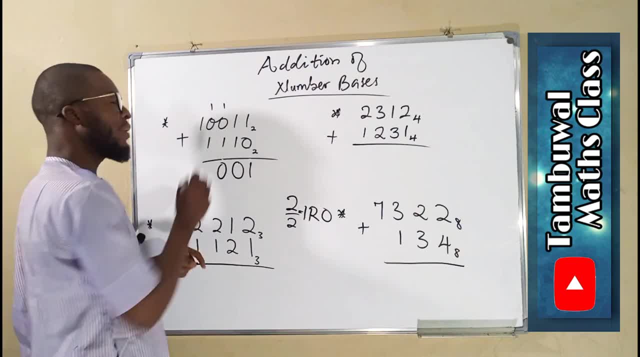 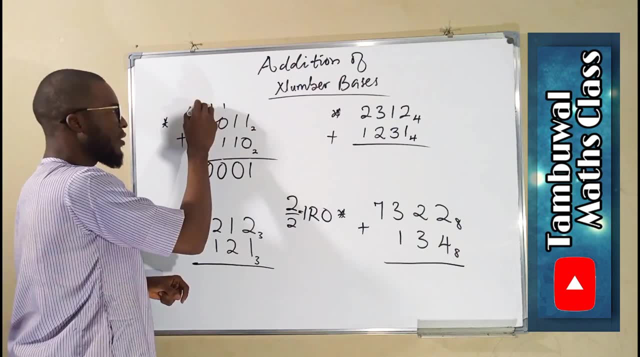 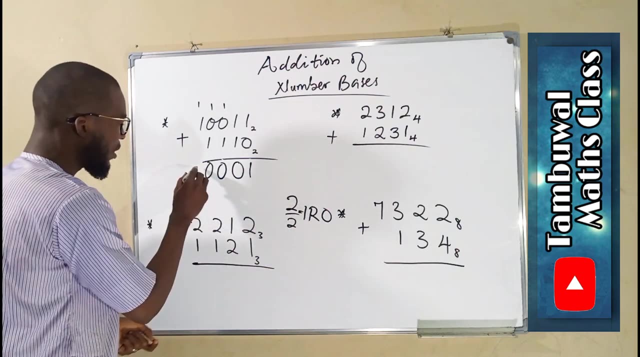 remainder. take that 1 to the next level. it also becomes 2: 0. you have 1 remainder 0: 0. you take 1 to the next number. 1 plus 1 is the same thing as 2. 2 divided by 2 is 1 remainder: 0- you're right here- 0. you take 1 to the. 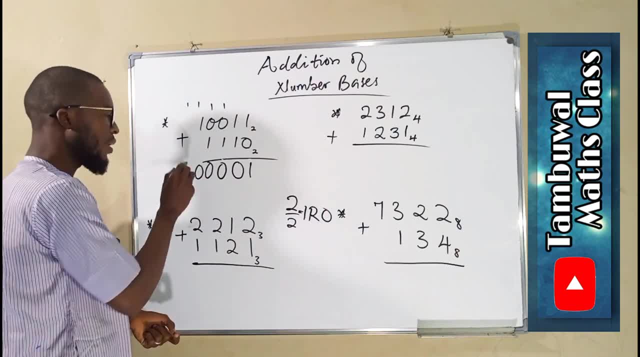 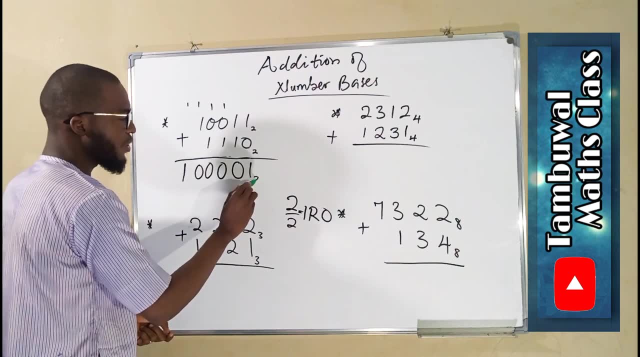 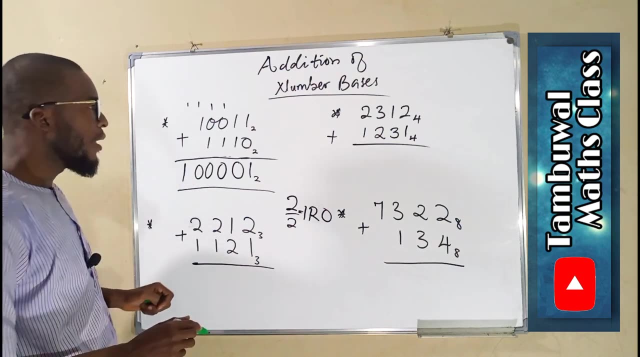 next, but we do not have any number to add with. then you drop it down. so these numbers are in base 2. if you add this and this together, you shall have 10 days. now let us move to the next one. we have all of these numbers in base four. 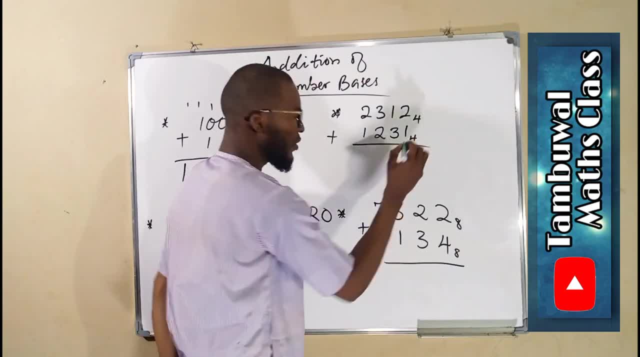 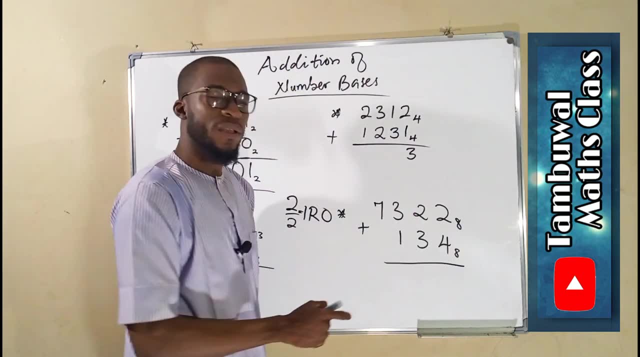 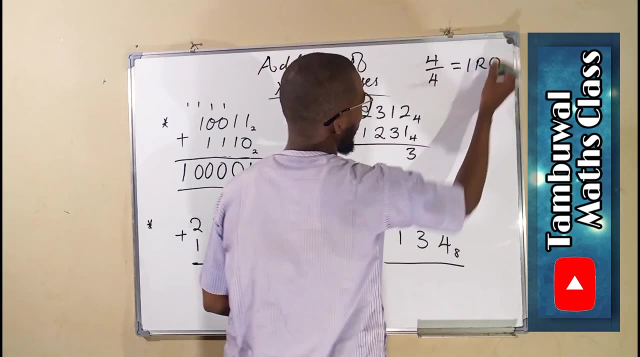 two plus one is three. we can write three because it is less than four. one plus three is four, but four is the same thing as our base. so we see four divide by four, which is equal to one remainder zero. so we write zero here. we take one to the next. 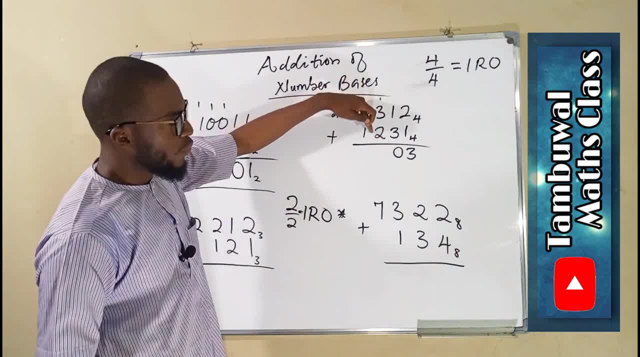 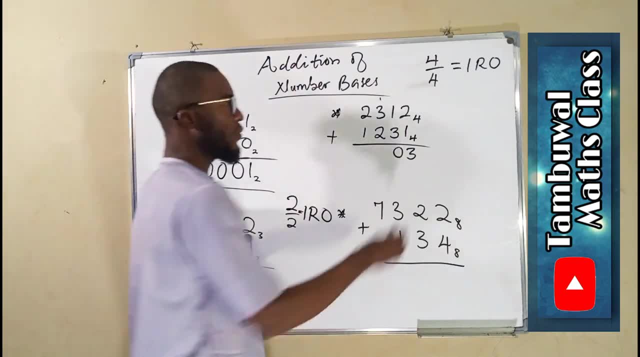 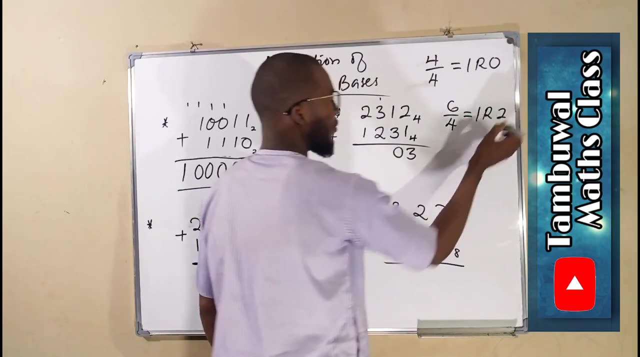 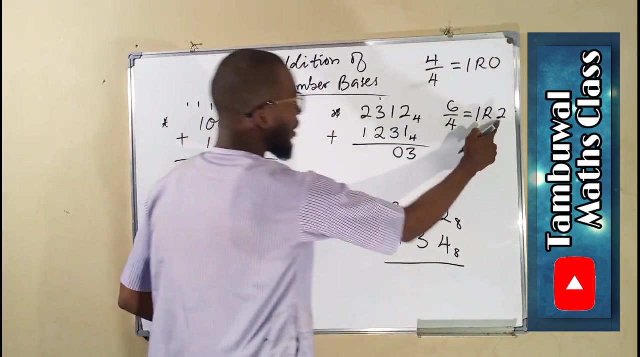 level. three plus two is five plus this other one, making six. six is greater than our base. so we say six over four. this is the same thing as one remainder two, because four can go into six only one time, but we have a remainder of two. so we write down the remainder and take that one to. 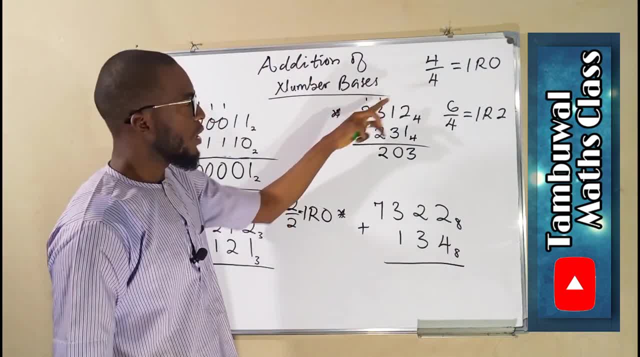 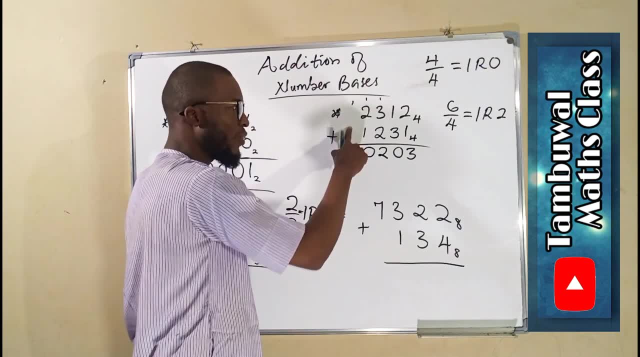 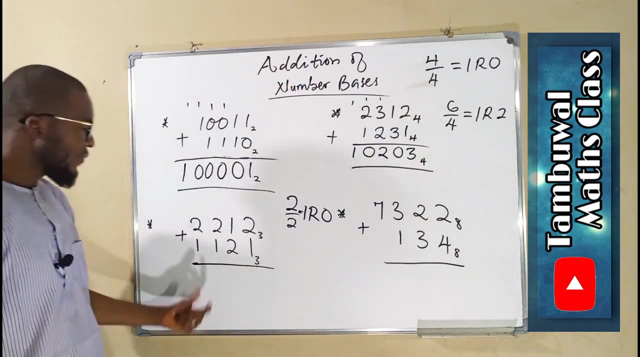 the next level. three plus one is three plus this other one, making four. and if you have four is one remainder zero. so we write zero, we take one to the next and that is not any number here, so we drop it down. this number is in base four. let's move to the second, to the last one. these numbers are all in. 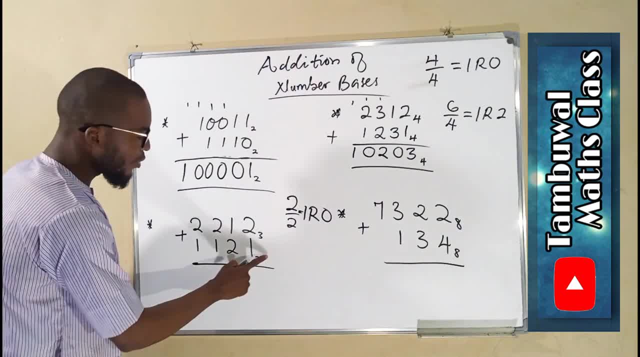 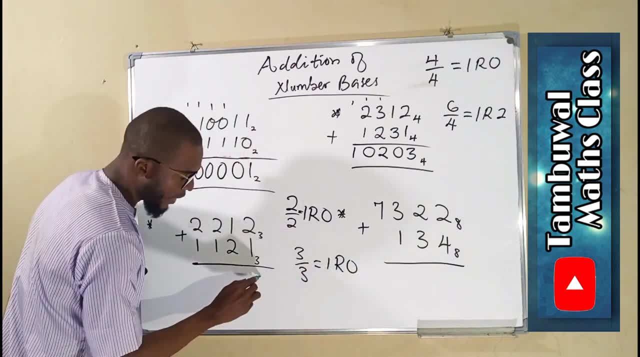 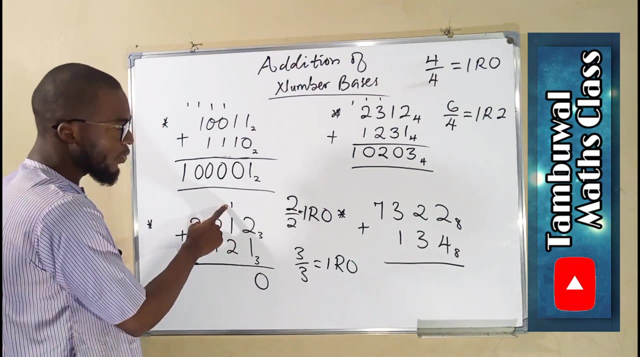 base: three, two plus one is three, and three is the same thing as our base. so we say three divide three, this is equal to one remainder zero. write down the remainder. take one to the next. one plus two is three, and three plus one is four. so if you have four, you see. 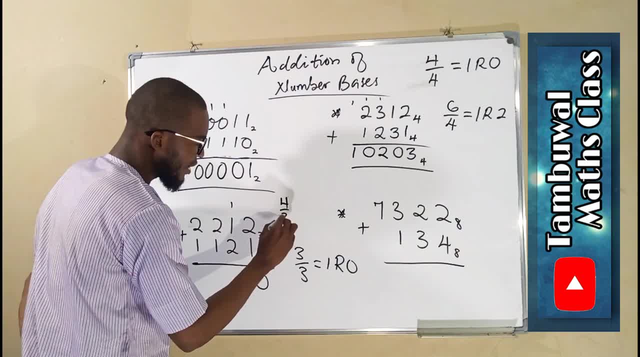 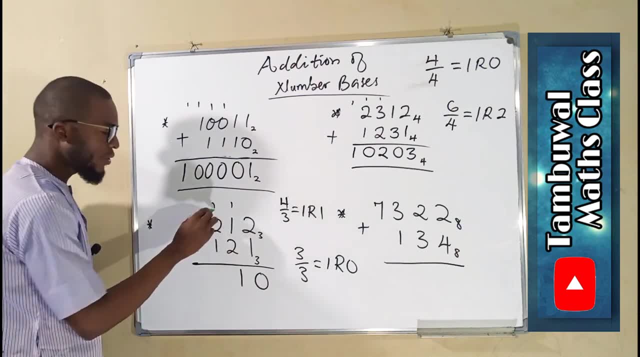 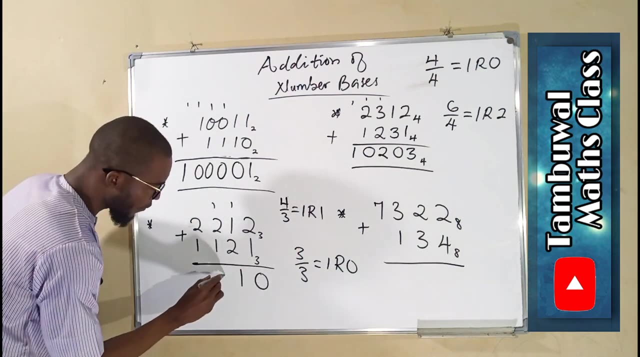 four divide three, this is equal to one, remainder one. write down that remainder. take that one to the next. two plus one is three plus one is four. the same thing. with this. we have one. we take one to the next. this plus this is three plus one is four. the same thing we. 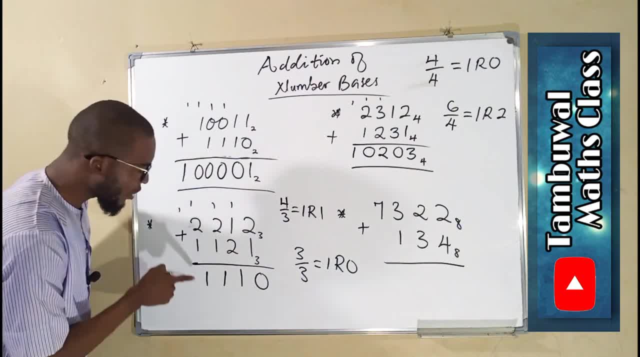 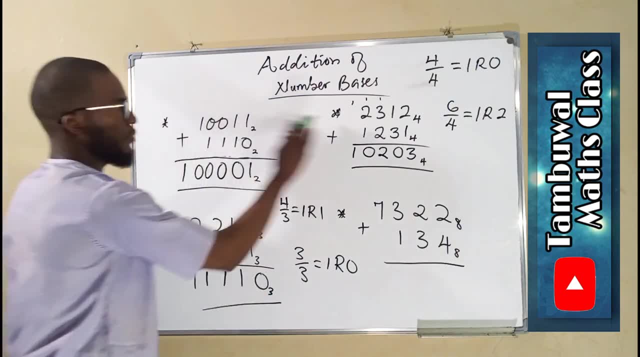 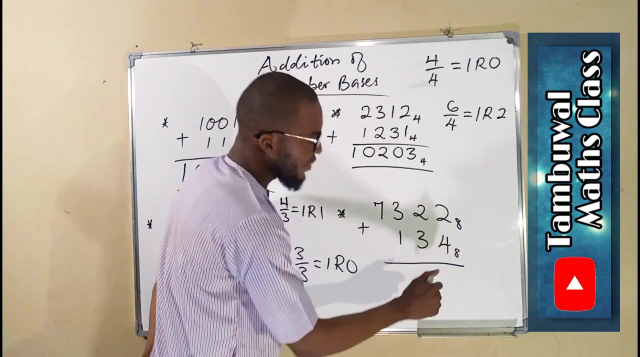 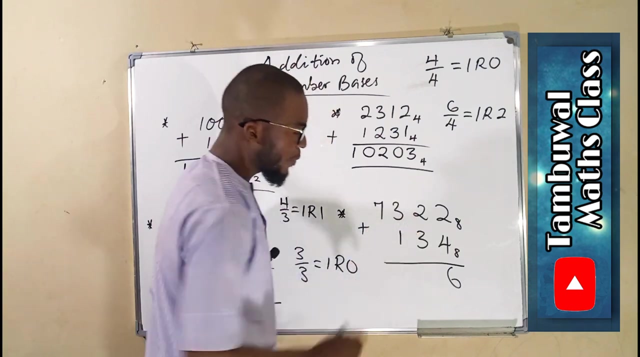 have one, we take one to the next, but there is not any number to add with you. drop it down. this is base three, the last one there in base eight. two plus four is six. six is less than our base, so we can write it um. two plus three is five, which is less than our base. we can write it also. 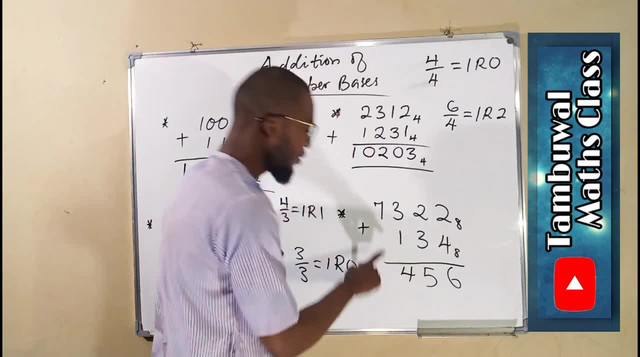 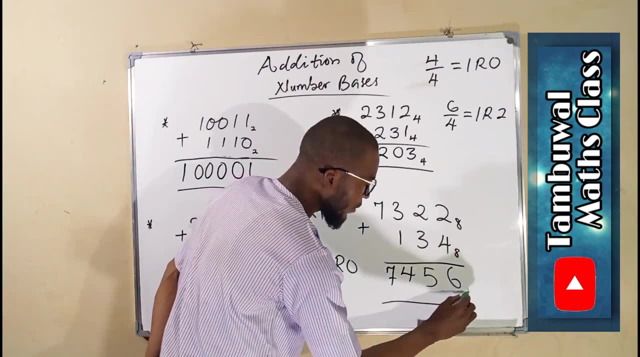 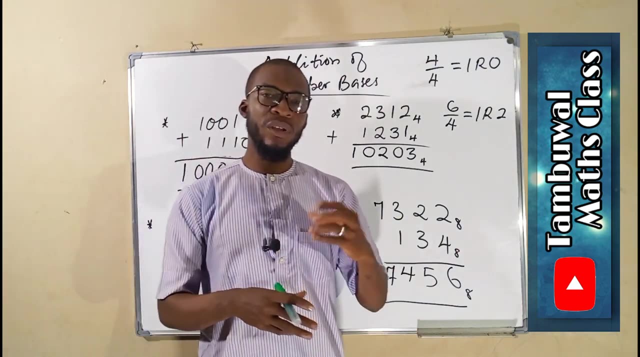 three plus one is four. we can write it as well. seven plus nothing is seven, and seven is less than our base. we write it down. so this is base eight. so this is how to add numbers in the same basis. in our next class we are going to see how we can add numbers that are in different basis.